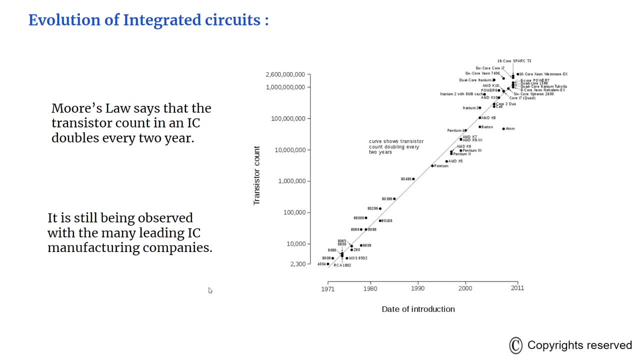 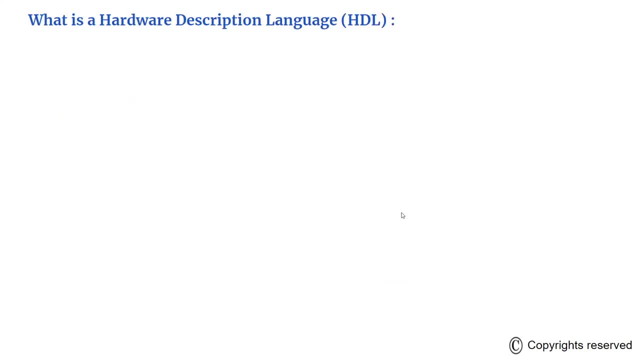 This Moore's law is still being observed with many leading IC manufacturing companies, for example Intel, Qualcomm, Nvidia, etc. What is a hardware description language? As you can see, the number of transistors in an IC is growing enormously, So the designers have moved from manual methods of doing to 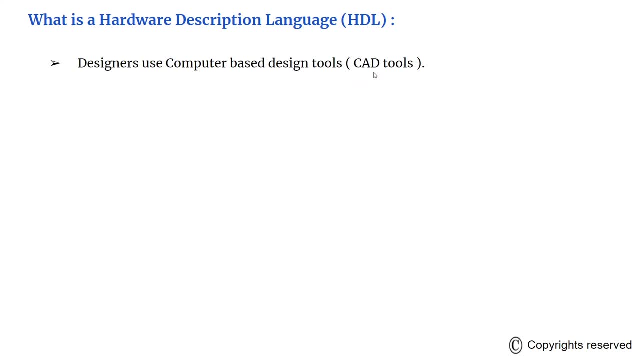 computer based design tools, called CAD tools. CAD means Computer Aided Design. For the computer to understand, it needs a separate kind of language. as you might know: C, C++, etc. So HDL is a language that describes the hardware. HDL stands for Hardware Description Language. 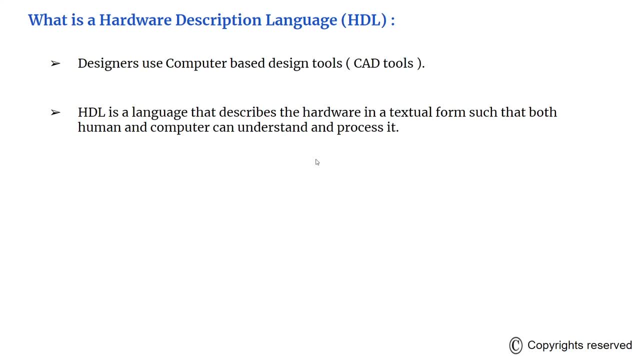 It describes the hardware in a textual form such that both human and computer can understand it and the computer can process and read it. In simple words, HDL describes the relation between output and input of a hardware block. For example, this is an OR gate, where the output is OR of A or B, the inputs. 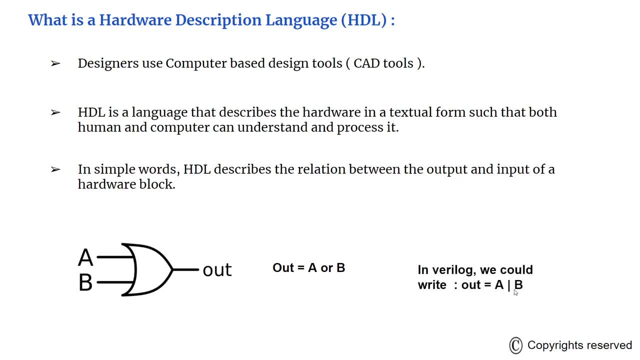 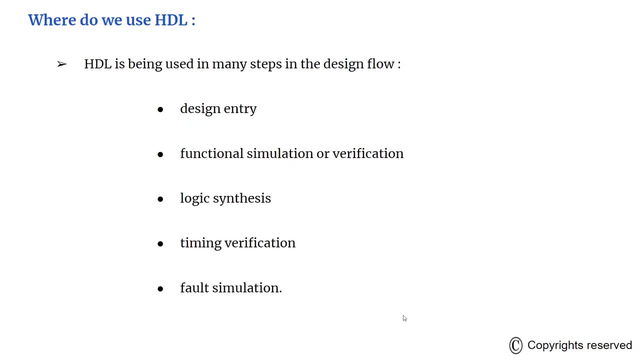 In a HDL verilog you would write it as OR equal to A or B in this fashion which the computer can interpret it. So we will learn about this in the next video. Where to be is HDL? HDL is used in many steps in the design flow of an integrated circuit. 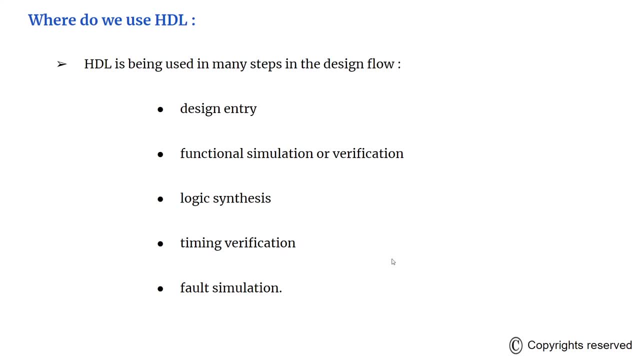 So these are some of the things, So we will try to get an idea of what this means In the next few slides. Design Entry creates an HDL based description of the functionality that is to be implemented in hardware. Depending on the hardware description language, the description can be in a variety of forms. 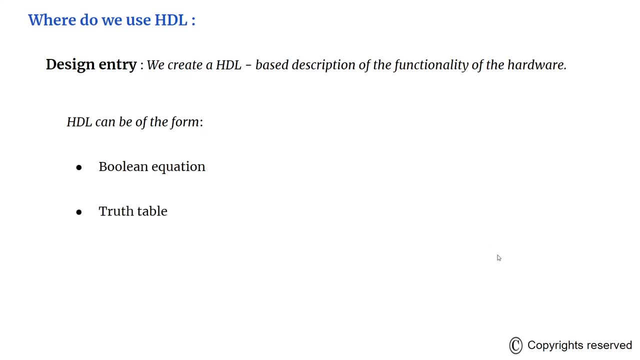 Boolean equation truth table an atrist of interconnected gates or it can be having the information about the interconnections between smaller circuits which neutralize the circuit. Logic Simulation: A simulator interprets the HDL and then generates the output that we can understand. 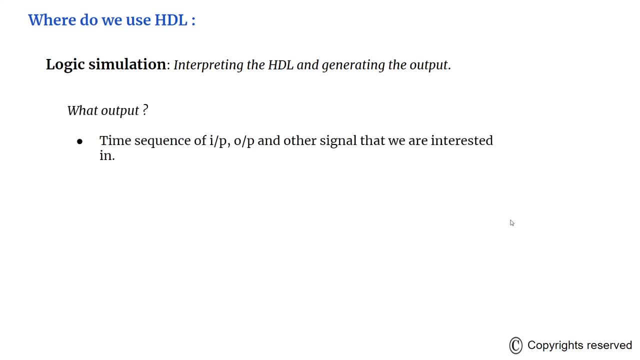 It can be of time-honored sequence of input and output values and other signals that we are interested in, Or it can be the waveform plot of the signals which we can read. So, with the help of logic simulation, we can see if the circuit is functionally correct. 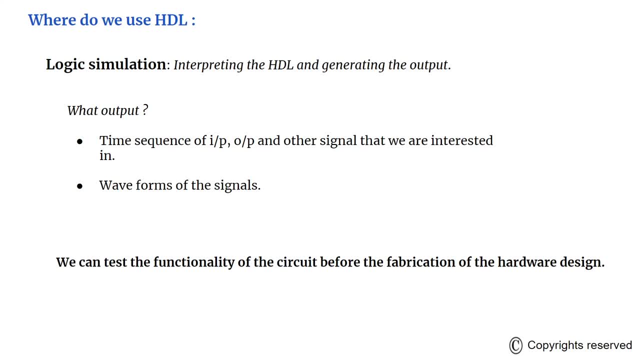 or no. We can also simulate errors in a design without having to physically create and operate a circuit. Errors that are detected during this stage can be corrected by modifying the HDL description that we have given To simulate a digital system. the design is first described in HDL and then verified by 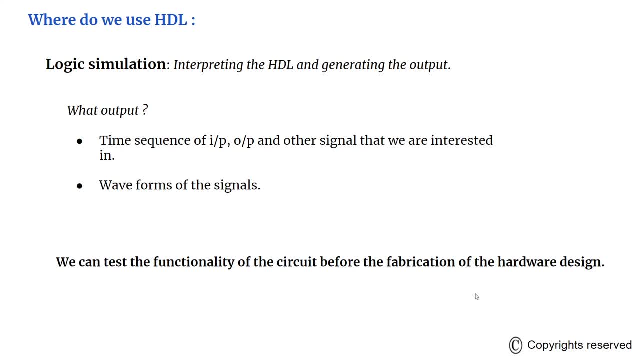 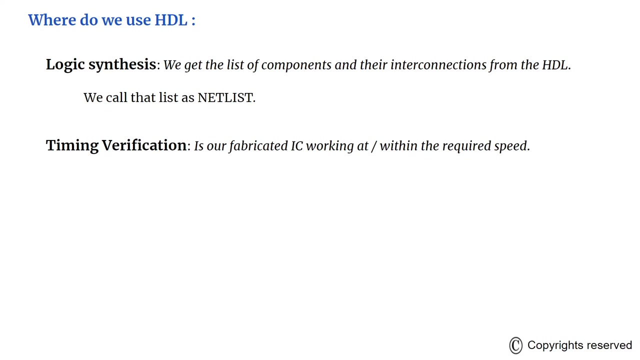 simulation, and then it is implemented. Logic synthesis is the process of deriving a list of physical components and their interconnections from the model to the system. That's what聽 successfully This method of orders the inputs. Watch this video now. – – – – purposes. against that, You may also buy these logical Untergradation systems. data. 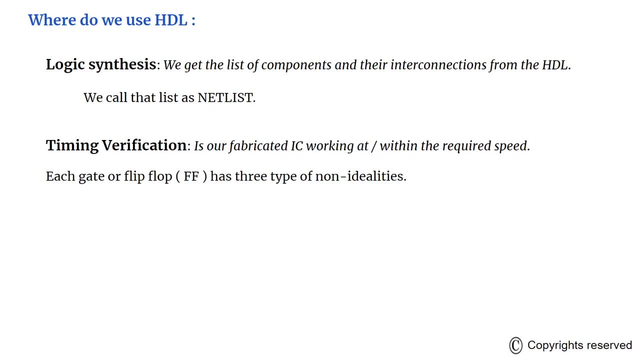 Ideal transition at the input of a circuit cannot immediately cause a change in the logic value at the output of a circuit. That is because of these non-idealities in the gate or the flip-throw. They are set-up time, hold time and propagation delay. 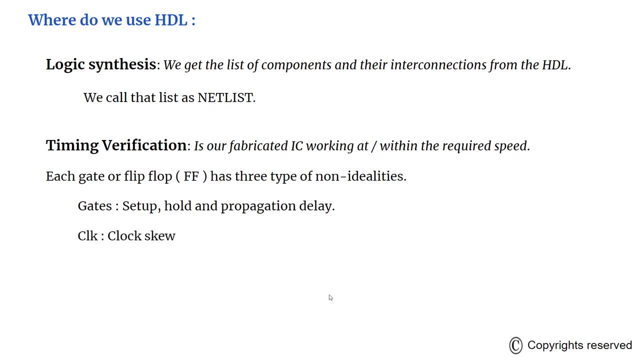 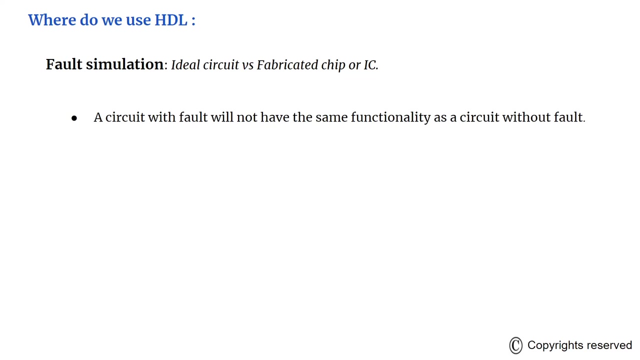 Clock has clock scheme Timing. verification checks each signal path to verify that it is not compromised by the propagation delay. Fault simulation compares the behavior of an ideal circuit with the behavior of a circuit that contains a process-induced flaw In the fabrication. the companies make sure the room is very clean. 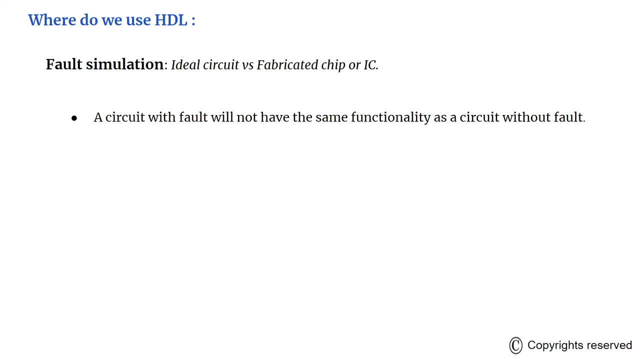 The dust and other particles in the atmosphere can cause a circuit to be fabricated with a fault. A circuit with a fault will not have the same functionality as a circuit without fault. The ICs that we have has only a fault: There are no edge pins available. 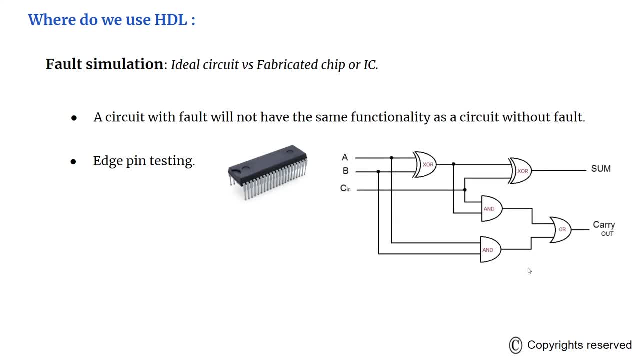 We only have access to inputs and outputs. This is a circuit that shows the full adder In the IC. we have the access to the inputs and outputs. We do not have access to the intermediate nodes or the wires. Suppose there is a fault that is induced during the fabrication.